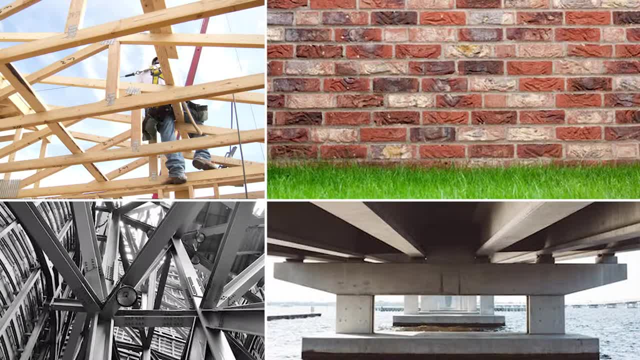 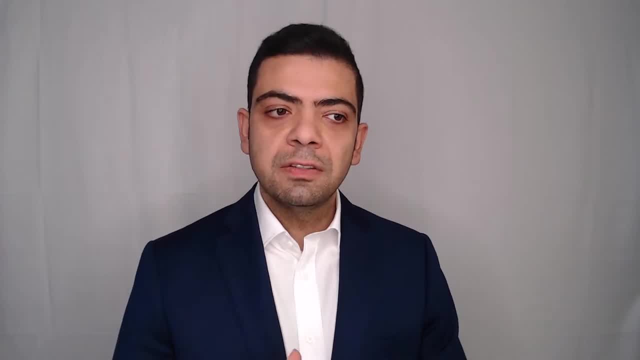 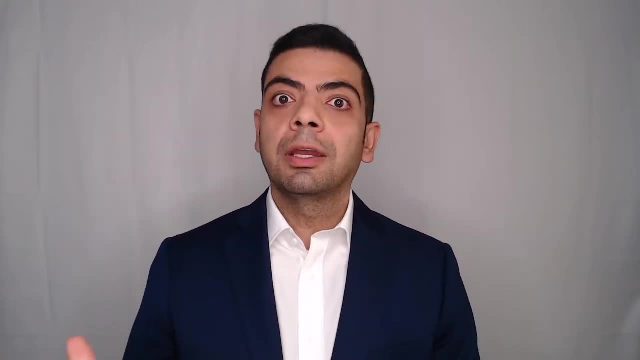 steel, structural steel, reinforced concrete, masonry and wood. So I want to take you through each material: what's the pros and cons and what would be a good application for each one of them. and I also want to touch on like the manufacturing industry of these building materials and how. 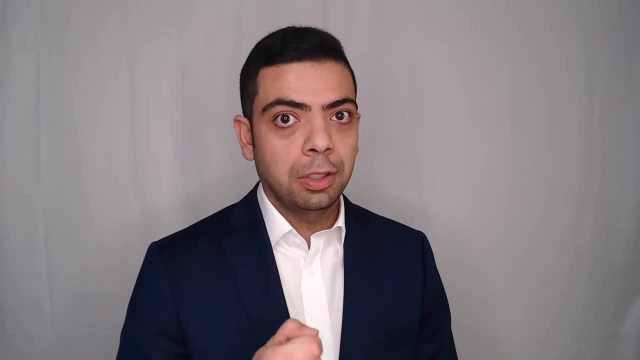 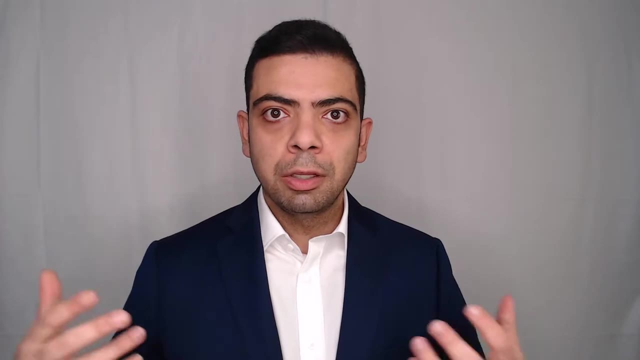 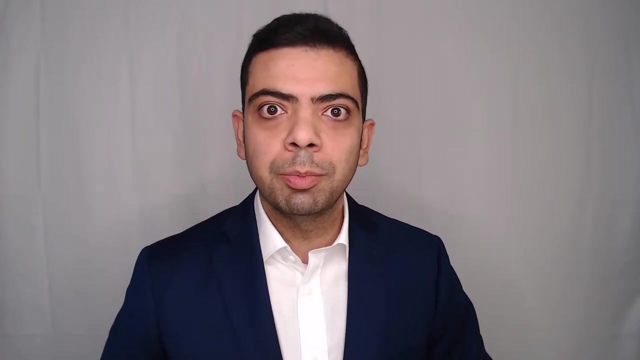 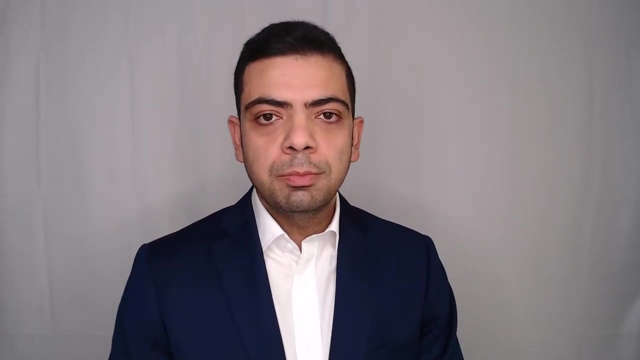 important to do testing and control the quality of these materials so it's reliable and sustainable. everyone involved in the construction industry can rely on a steady source and supply of building materials so we can keep on growing our cities and build more buildings. So let's start with a quick comparison between these four materials that I want to talk about. 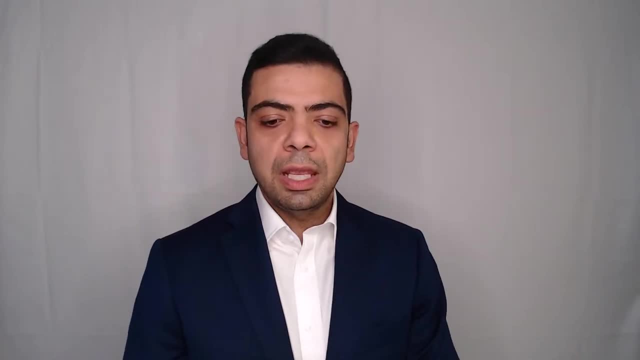 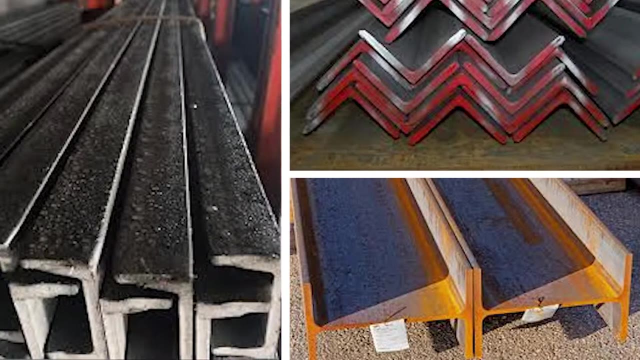 Steel. this is usually comes in structural shapes like angles or white flange beams or like steel. this is usually comes in structural shapes like angles or white flange beams or like C-channels. They're usually hot rolled steel sections and it's pretty strong These sections. 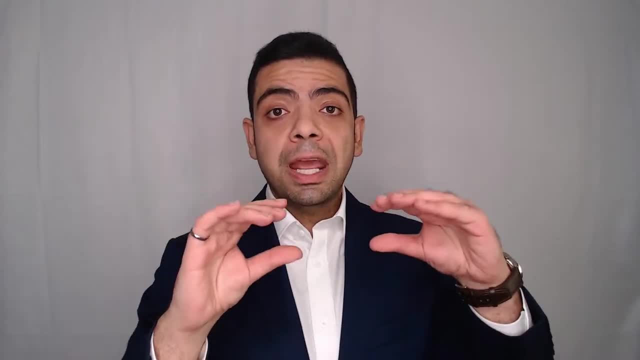 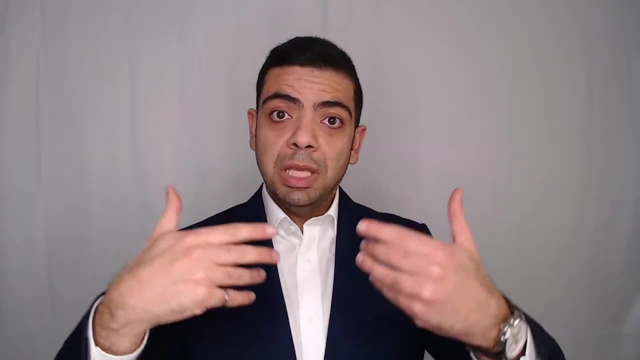 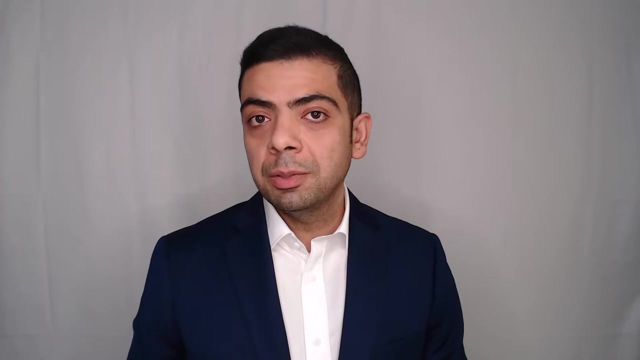 can be used together, can be welded together or can be connected using high strength bolts to create the framing of floors and columns and beams and basically stack multi-story buildings using these structural shapes. The other material I want to talk to you about is reinforced concrete. 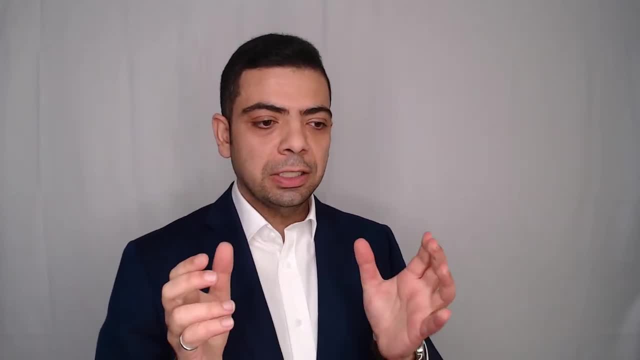 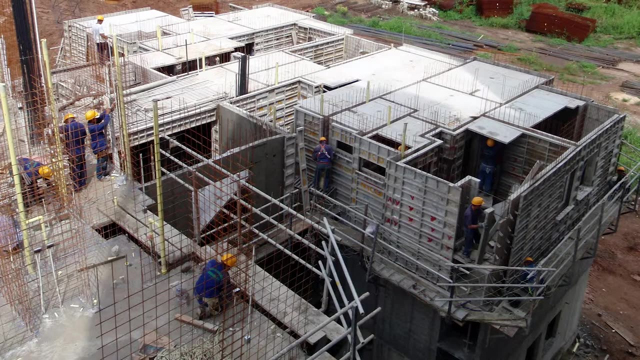 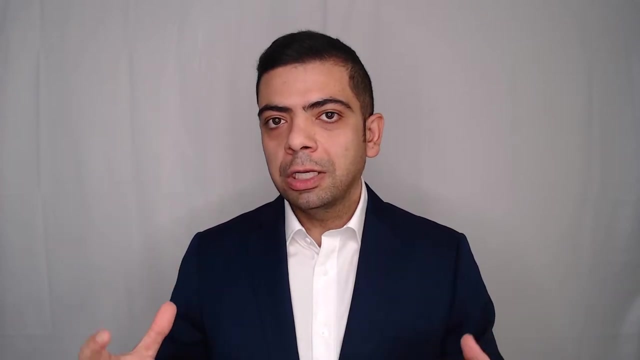 Reinforced concrete is very versatile. It basically uses formworks that you can shape it the way you want fresh concrete to look like, after it hardens and cures, and then you pour concrete into it. and it takes time for fresh concrete to harden and to gain strength, usually about seven days. 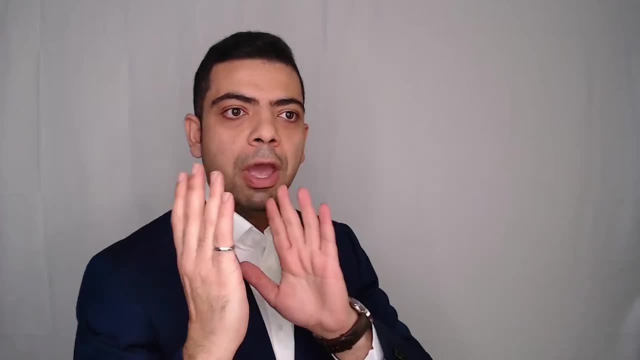 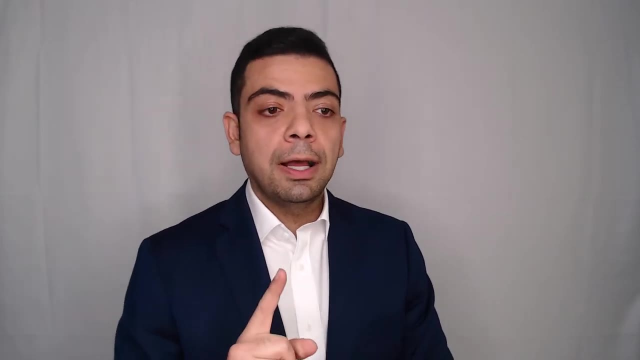 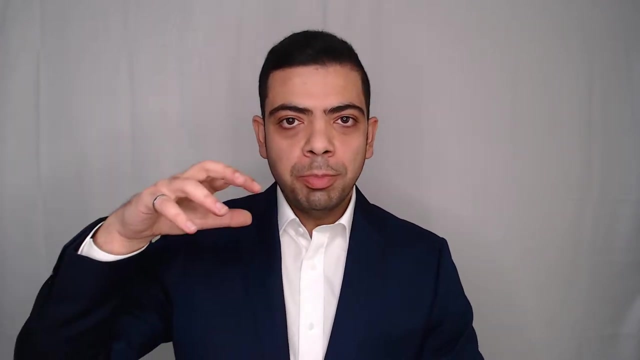 And after seven days you can remove all the formworks and now you have the shape of the concrete in, like a stone-like hard material. There are some weak points when it comes to concrete. It's very good in compression when you load it in compression. 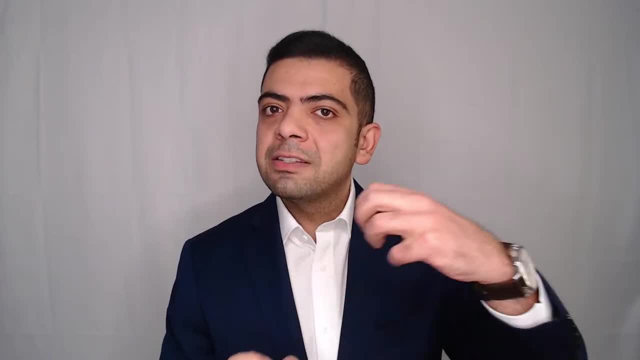 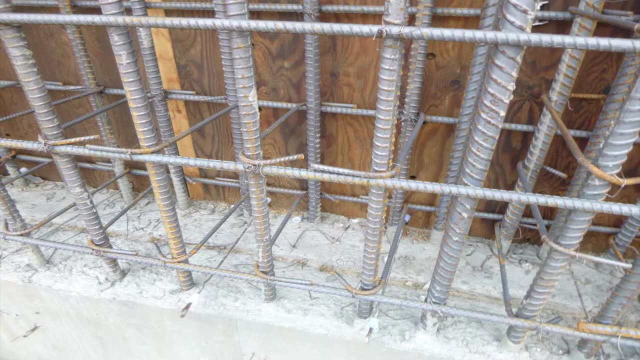 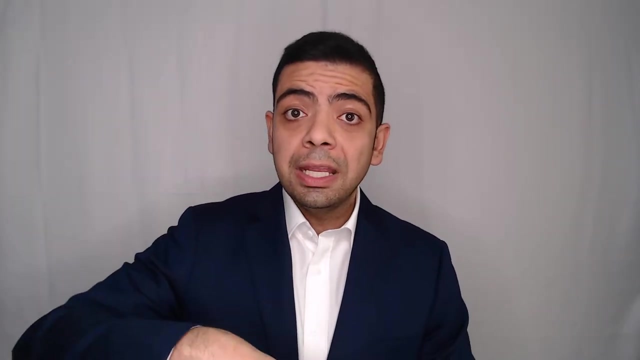 but it's brittle and doesn't have a lot of tensile strength. So combining it with internal rebar or steel reinforcing gives it creates this sort of new composite material, reinforced concrete or reinforced concrete, With excellent properties in both tension and it can in both compression and it can take tension as well. 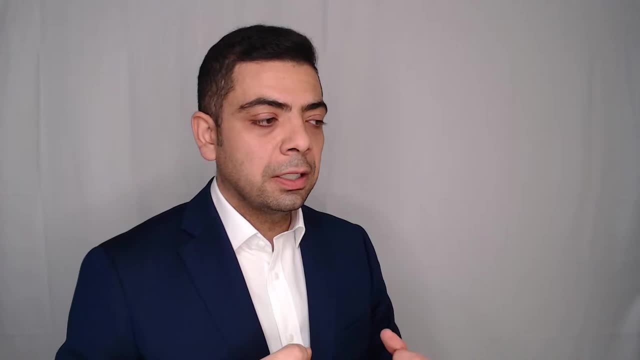 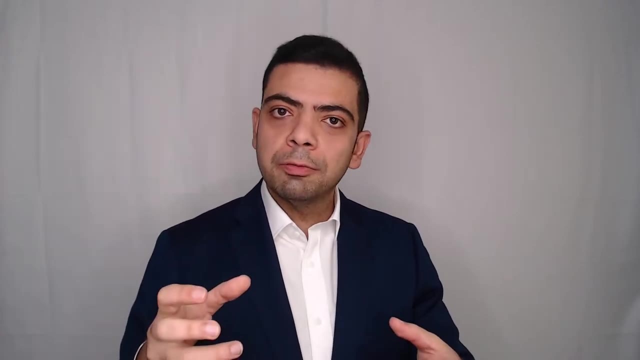 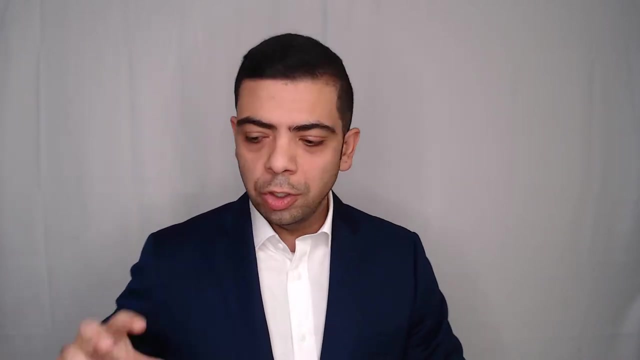 When it comes to masonry, masonry is basically wood. cement blocks made out of concrete are very popular, very used widely. A lot of builders and contractors. they like them because they're easy to work with. You can use the units. you can think of it like as building with lego: you can put the units. 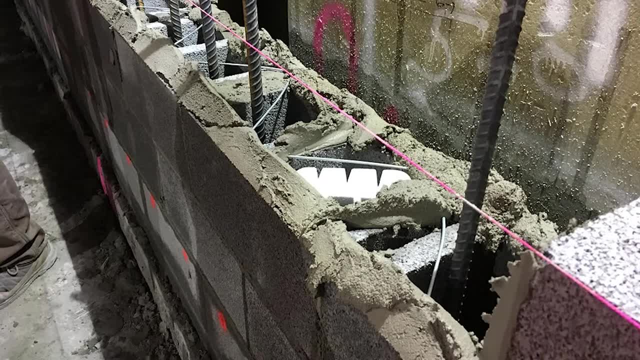 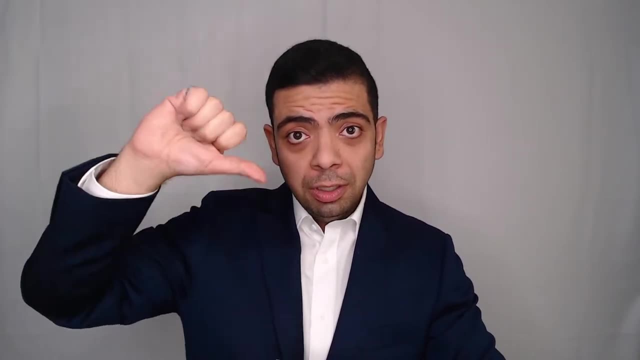 in here that are made out of concrete. This is a very good one. It takes mortar in between each layer and the cores or the voids of the masonry blocks. those can be reinforced. so again, that's the advantage of adding the steel rebar for tensile strength. It can be added after building a wall. 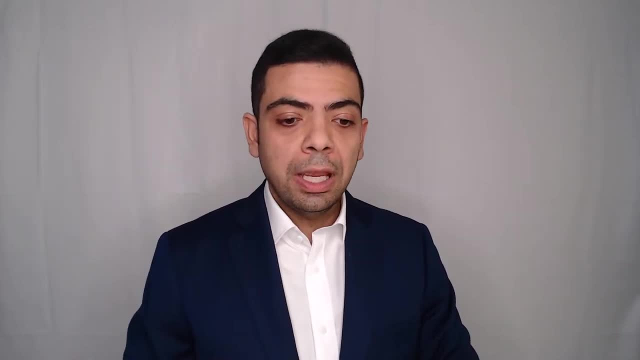 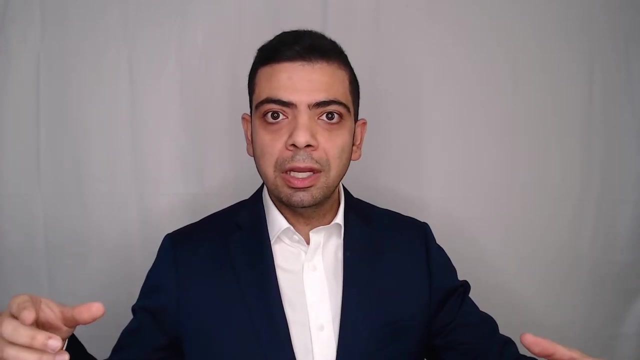 and cored so that improves the strength of the wall and this way makes the masonry a very versatile application. Usually it's done with it's used in walls. have with no cores filled all the voids or all the cores. have no reinforcing in it or you can fill. 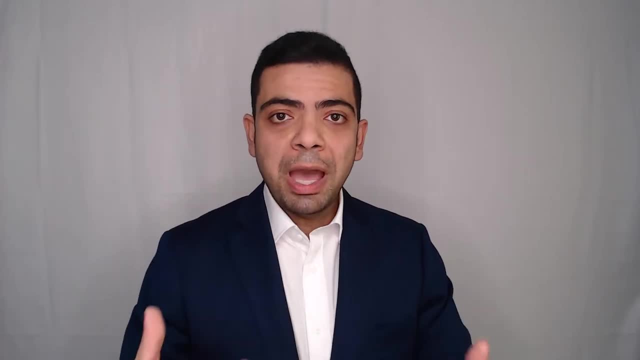 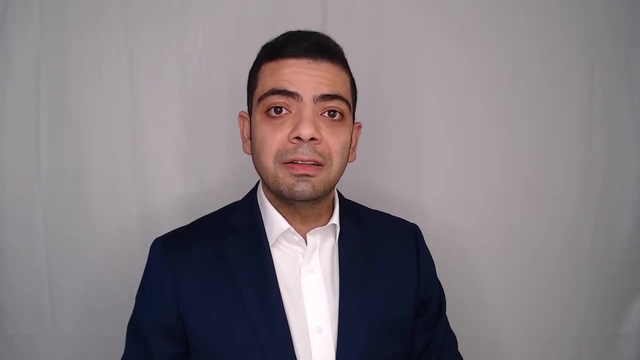 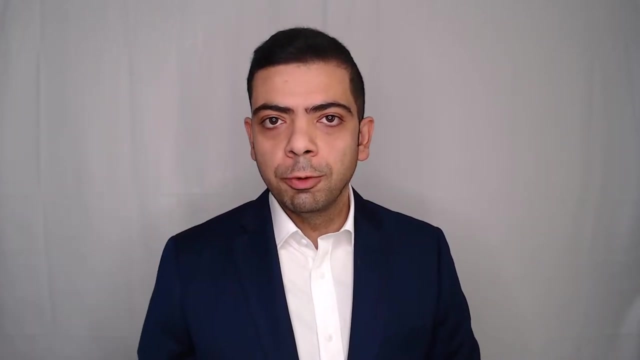 all the cores so that gives you a wide range of capacity or strength you can get out of masonry. the other material i want to talk to you about is wood. so wood obviously is a natural material. like there are different species of wood, it depends on the type of tree or the species of wood. 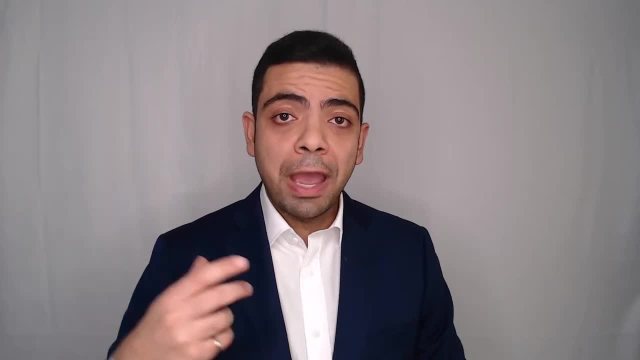 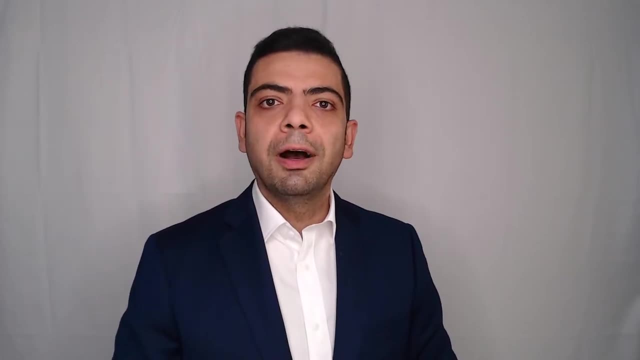 that it's manufactured from. obviously it needs to go through a process of curing or treatment to make the wood dry and suitable for structure application. and there are actually very good advantages to working with wood: it's light, it's easy to work with, it's ideal for short buildings. 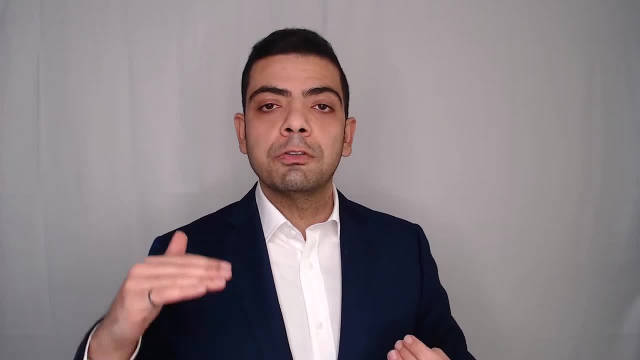 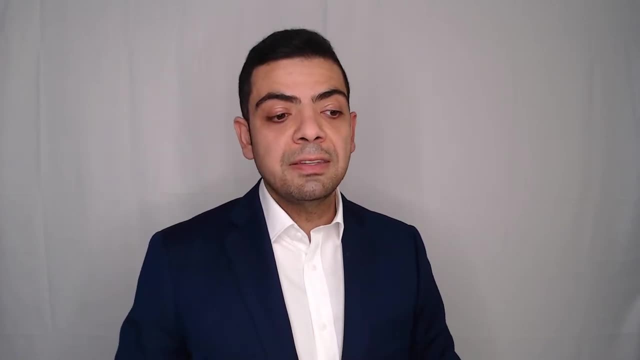 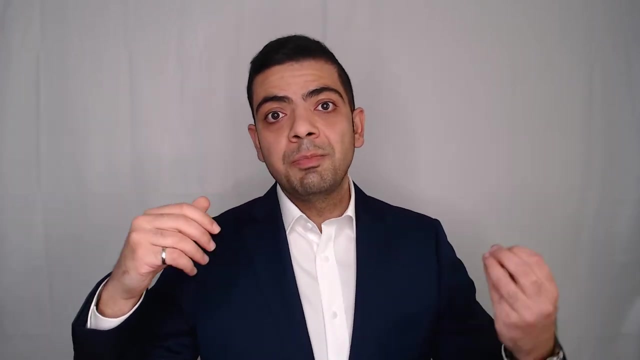 like. it doesn't work very well for, like, when you start stacking up multi-story buildings, there is a limit to how much you can build something like that from wood, but at the same time, wood has a very reasonable compressive strength and tensile strength as well, so this makes it a good application for roof trusses.